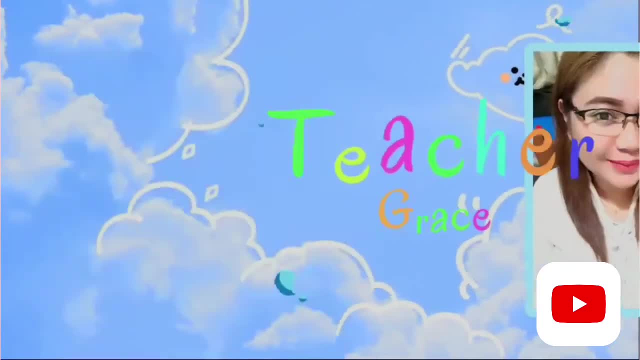 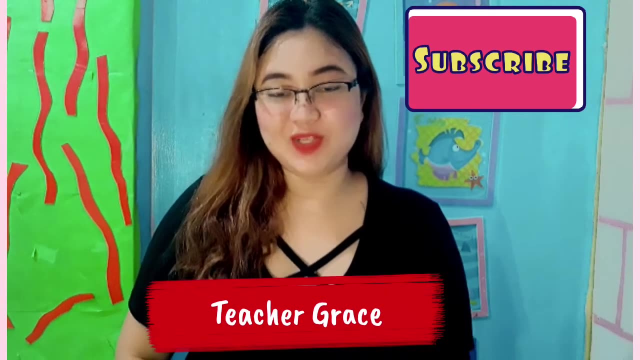 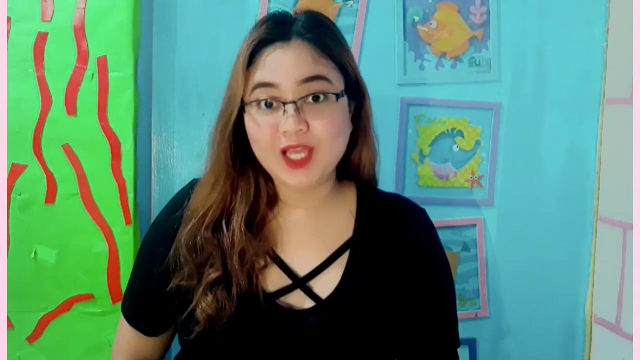 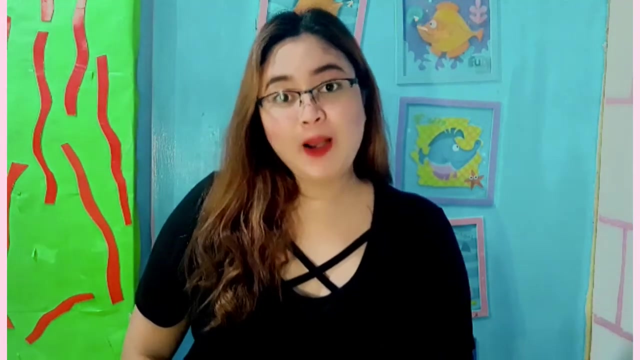 Hi everyone, I'm back. I'm Teacher Grace from Dominic Elementary School. How are you today? Hope you're fine, because for today's video, we are going to study about the four basic shapes. Yes, four basic shapes. Do you have any idea? what are those shapes? 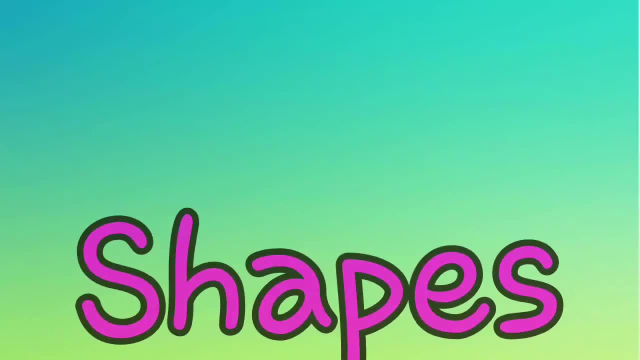 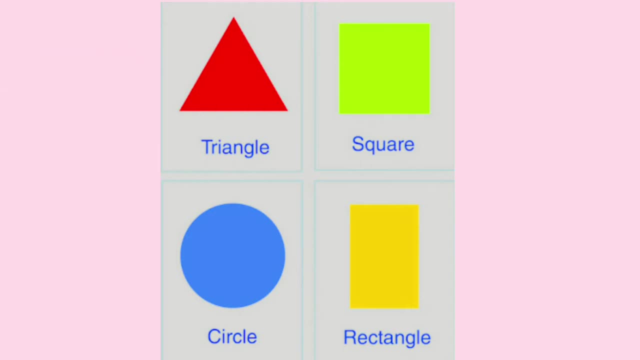 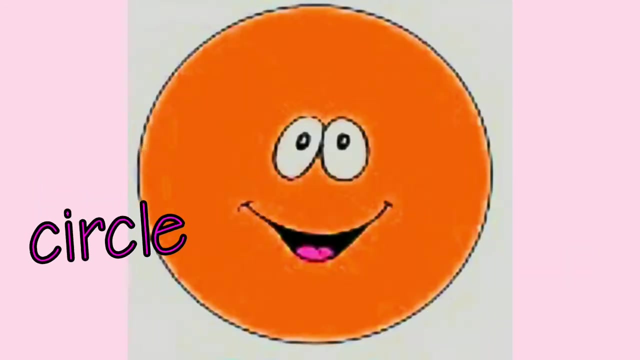 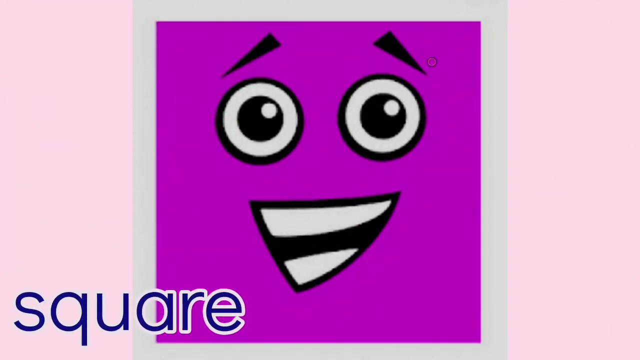 Let's see if you're right. Here are the four basic shapes: Triangle, square, circle and rectangle. This is a circle. It has no sides. This is a square. All its four sides are equal. This is a triangle. 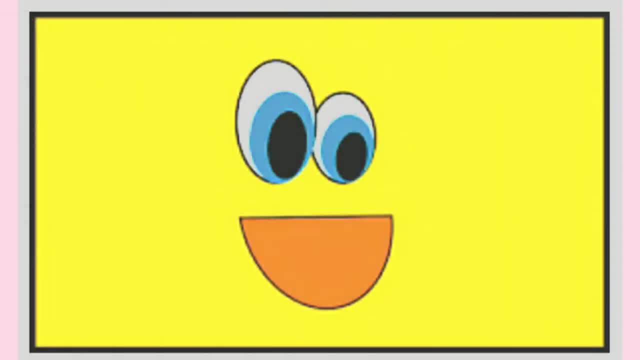 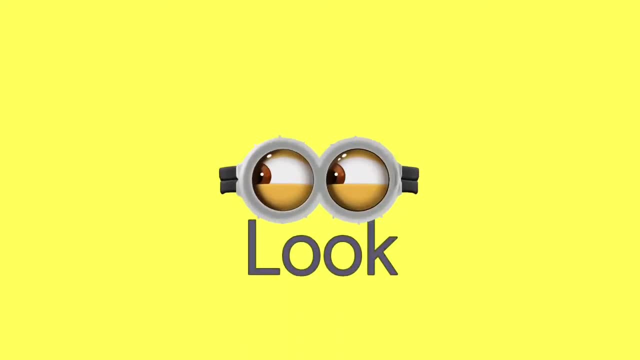 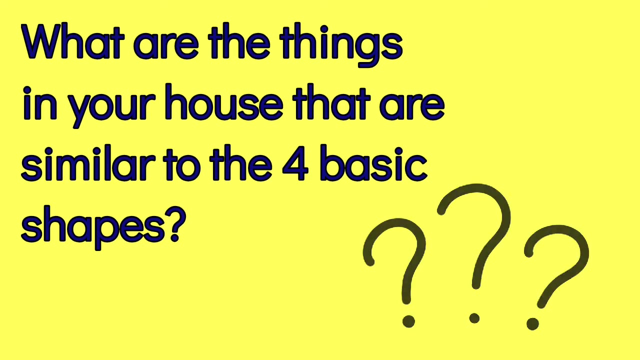 It has three sides And this is a rectangle. It has two equal long sides and two equal short sides. Look inside your house. What are the things in your house that are similar to the four basic shapes Done? I have some examples here. Please repeat after me. 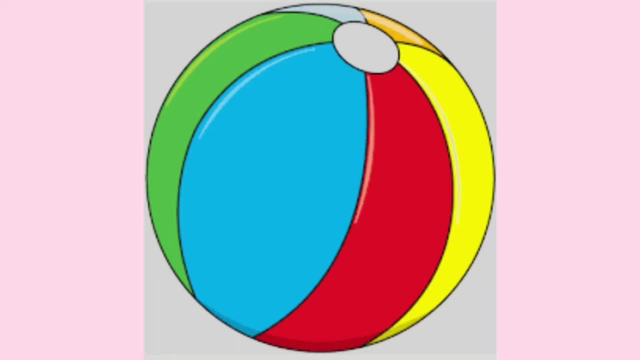 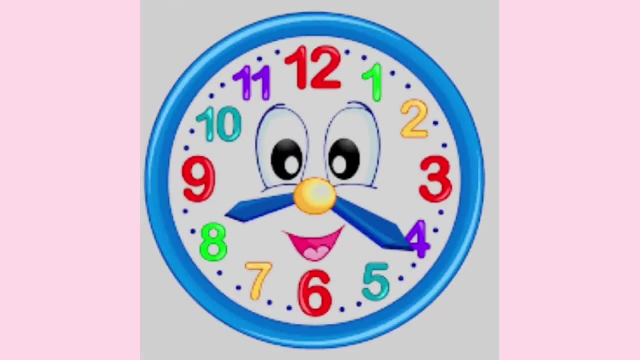 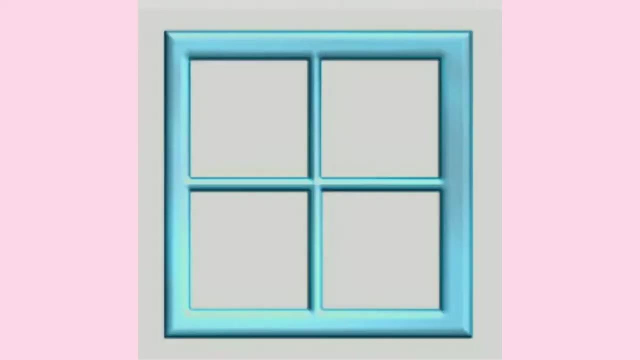 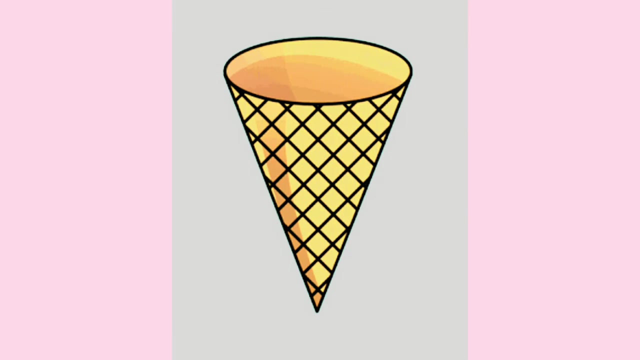 For the circle. I have here a round ball, Whole pizza And a round clock. For square I have a box Gift And window Window. For triangle I have a slice of cake, Pizza, An ice cream cone. 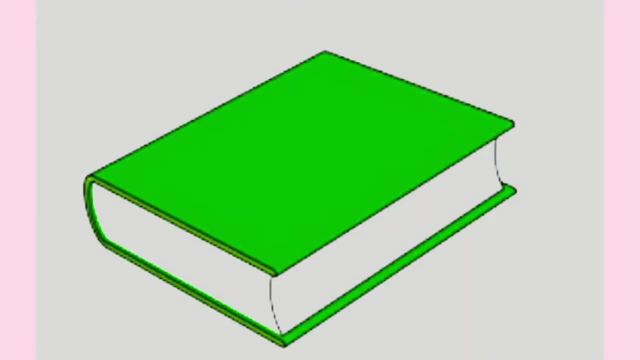 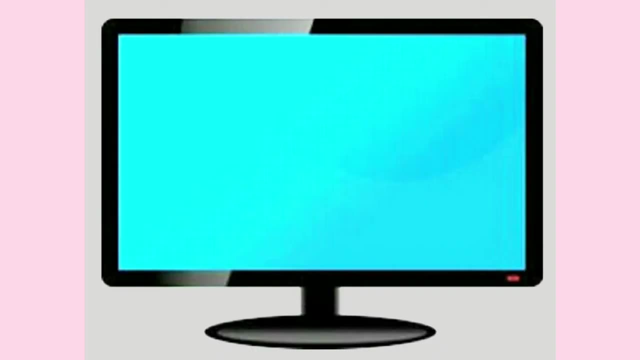 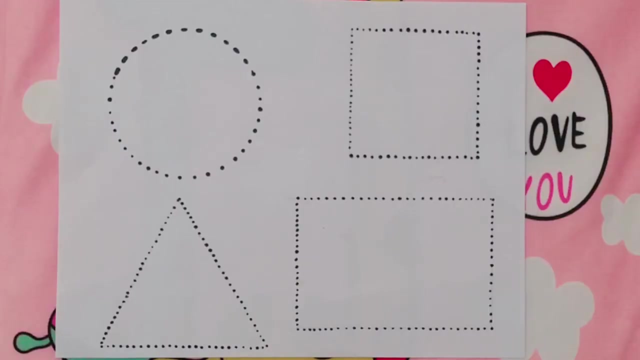 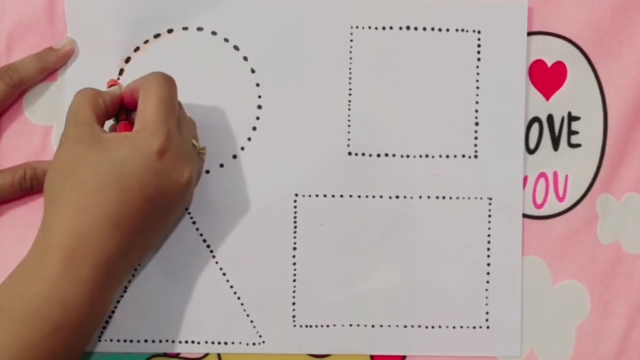 And a slice of pie For the rectangle. I have a book, Door And television. Now I'm going to teach you how to draw shapes by tracing the dots. First is a circle. You just have to trace the dots or broken lines. 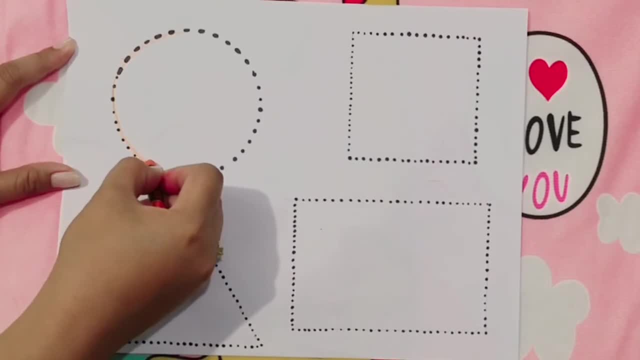 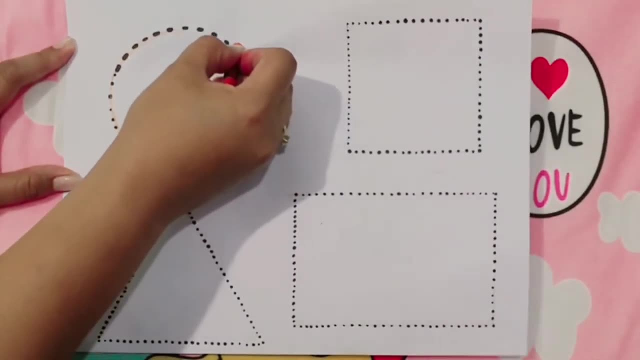 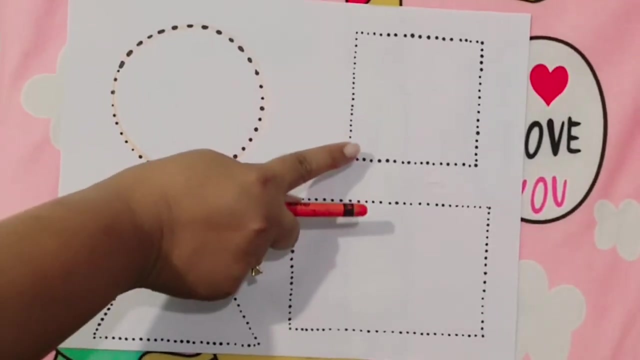 All you have to do is you need to control your hand. Done Next is square: Make a straight line down, And then you have to draw a square. Make a straight line down, And then you have to draw a square.